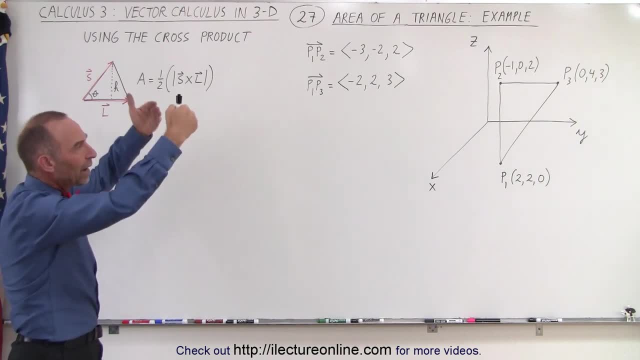 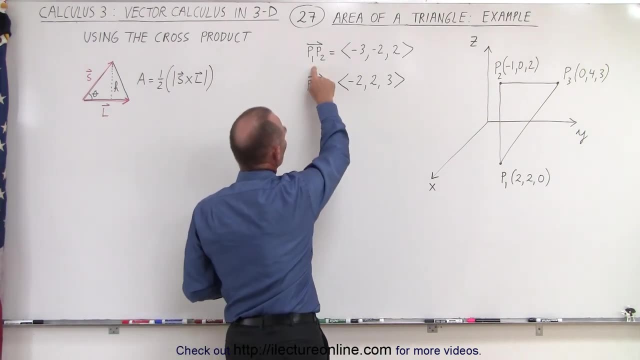 Now imagine this is not exactly in the YZ plane. It could be oriented in any given direction. And to help us out a little bit, notice that I've defined two vectors: the vector from 0.1 to 0.2, this way, and the vector from 0.1 to 0.3. 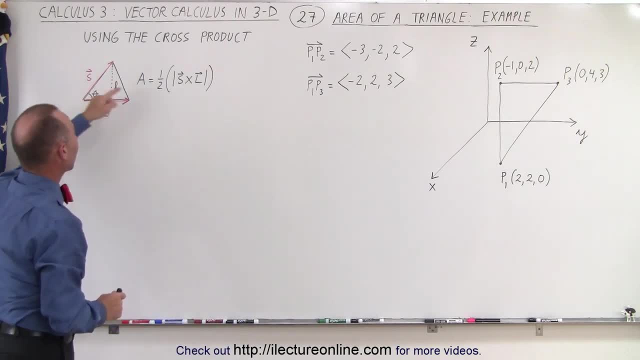 Now remember that from a previous video we realized that the area of a triangle can be found by taking one-half times the magnitude of the cross product of the base of the triangle, times one of the sides. But then it turns out with a triangle. it doesn't really matter, since we're looking for the magnitude only. 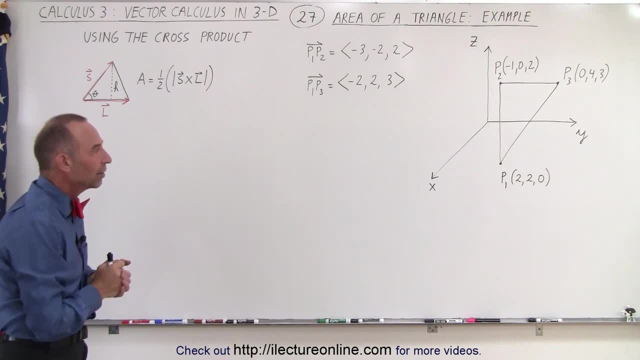 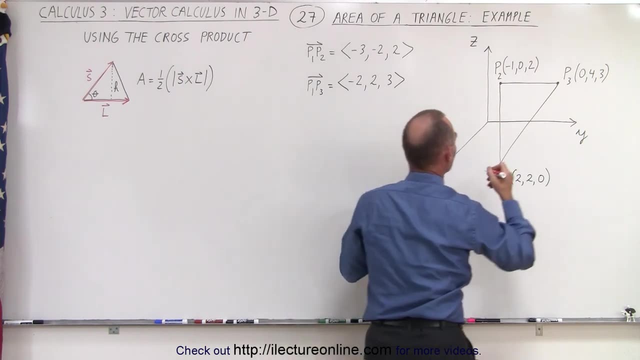 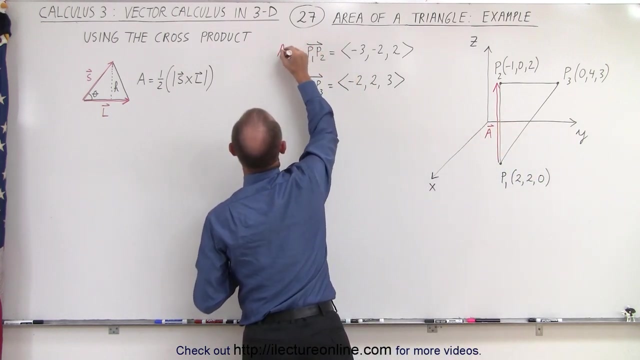 We can take the cross product of any of the two sides. So what we're going to do here is we're going to define the vector A from P1 to P2.. So this would be called the vector A. And so here, this is the vector A. 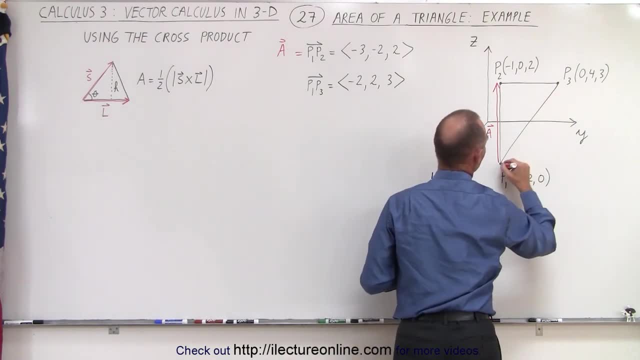 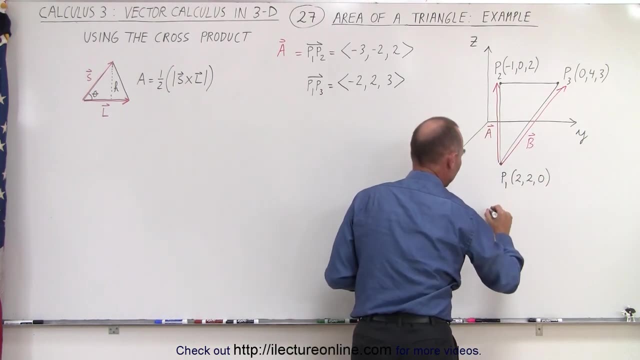 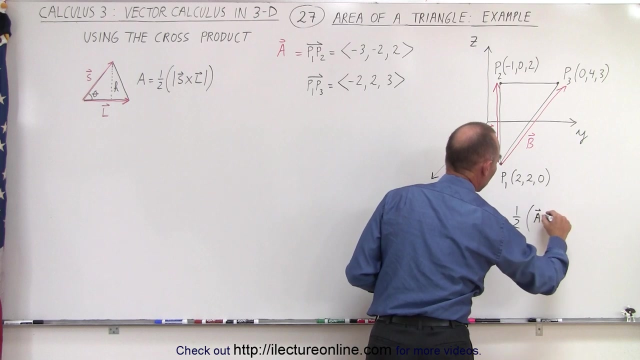 And we're going to define the vector B from P1 to P3.. And there's our vector B, And it turns out we can find the area just as well by saying that the area of the This triangle is going to be equal to one-half the magnitude of the cross product of two of the three sides of the triangle. 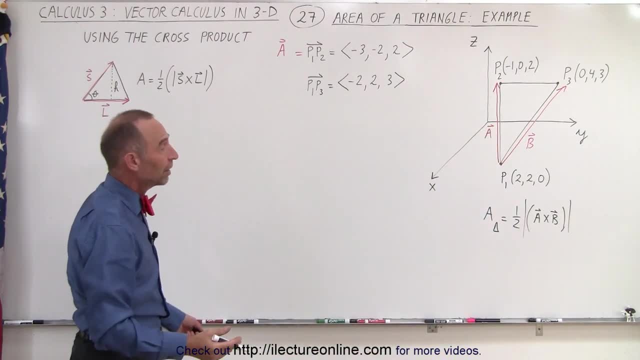 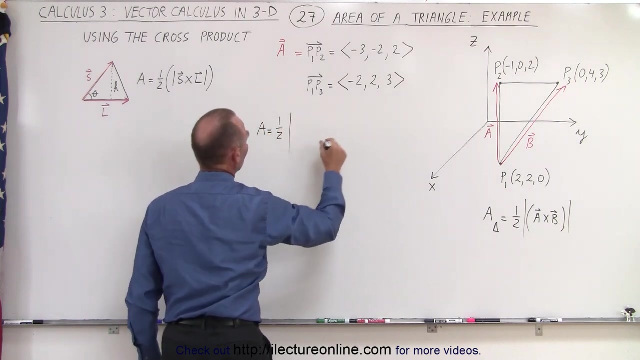 Like that, And so that makes it easy. Pick any two sides, express the two sides in terms of vectors. take the cross product and then multiply times one-half. Let's go ahead and try that. So the area is therefore going to be equal to one-half times the cross. 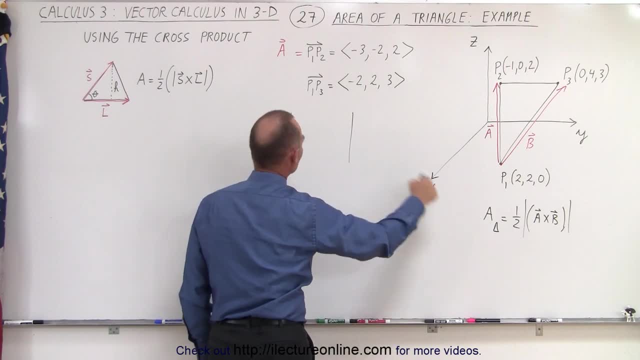 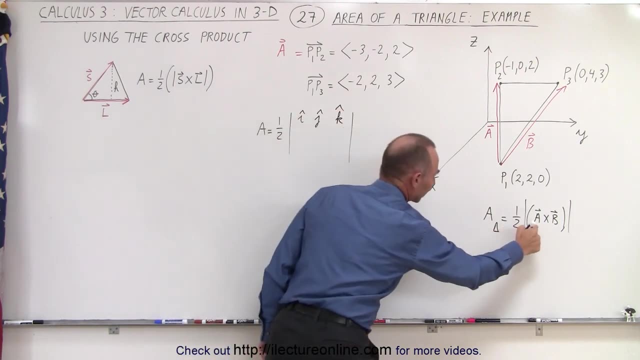 So this is the cross product of A, cross B, And so we have one-half, We have I J K. Now we need the components of the first vector A, The first vector A. Now, of course, I didn't do this one yet. 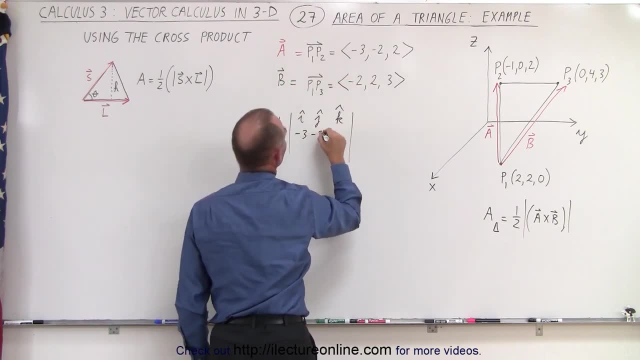 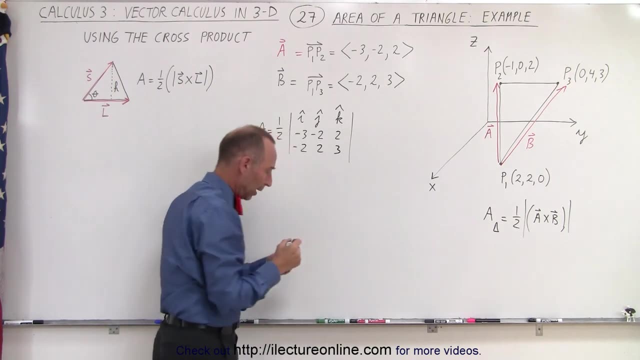 There's my B vector. That would be minus 3, minus 2, and 2.. And here are the components of the second vector, B, minus 2,, 2, and 3.. How do we find these components? 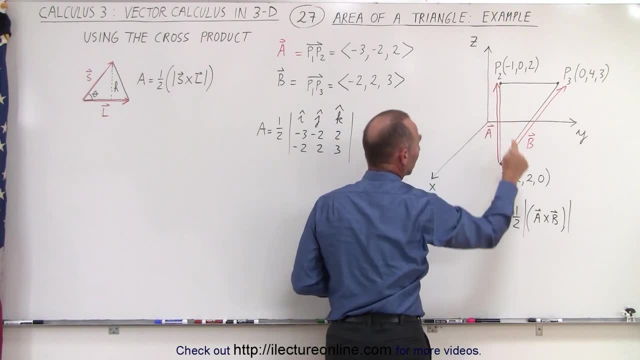 Notice that if we go in the X direction, from point 1 to point 2, we go from point 1 to point 2.. So from a positive 2 to a negative 1, that's a negative 3 change. From a positive 2 to a 0, that's a negative 2 change. 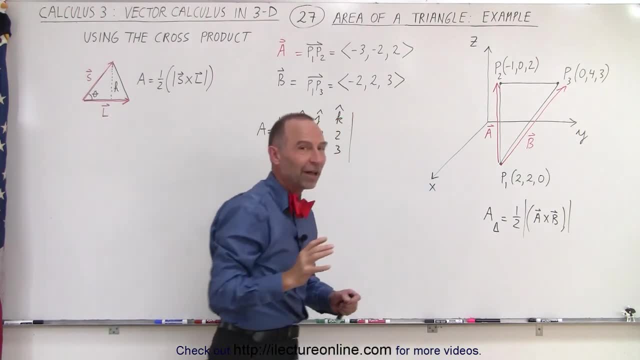 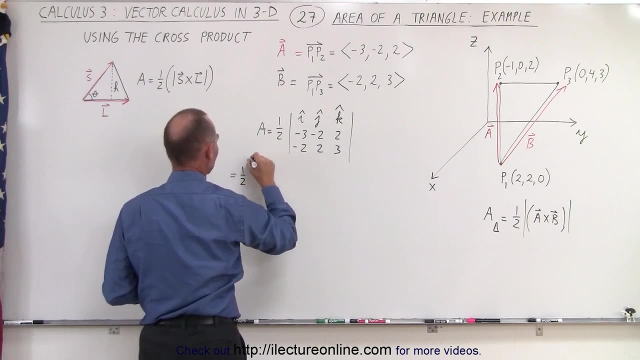 From a 0 to a positive 2,. that's a positive 2 change. So that's how we found the vectors. Now let's go ahead and do the cross product. So this is equal to one-half times I multiplied times negative 2, times a positive 3, that's a negative 6,. 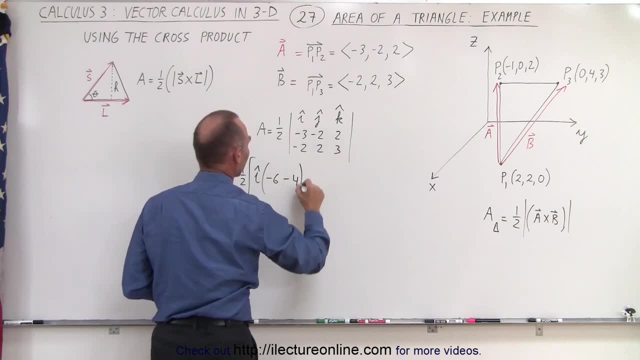 minus a 2 times 2,, which is 4.. And that would be minus J- whoop, that should be a J here. times we have a negative 3 times a positive 3,, which is negative 9, minus a 2 times a negative 2, that gives us a plus 4,. 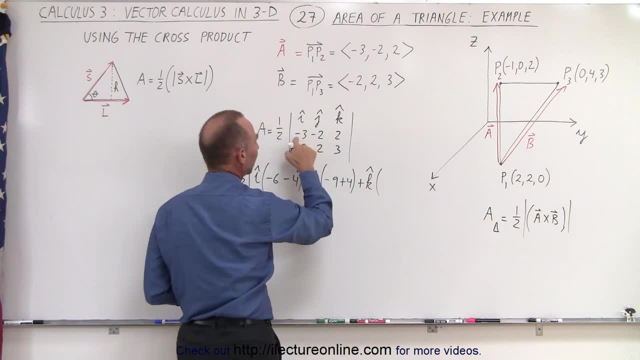 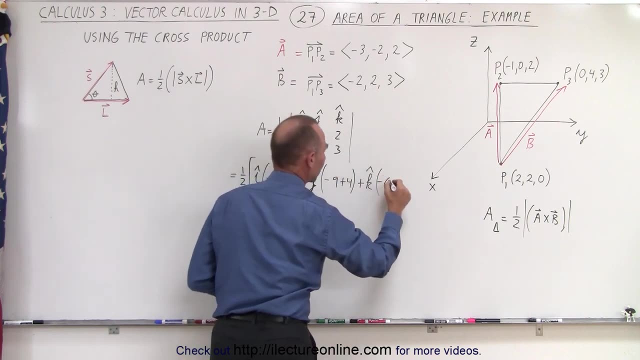 and then plus K, multiplied times a negative, 3 times 2, that's a negative 6, and minus a negative 2 times a negative 2, that's a positive 4, but we have to subtract, that gives us a negative 4.. 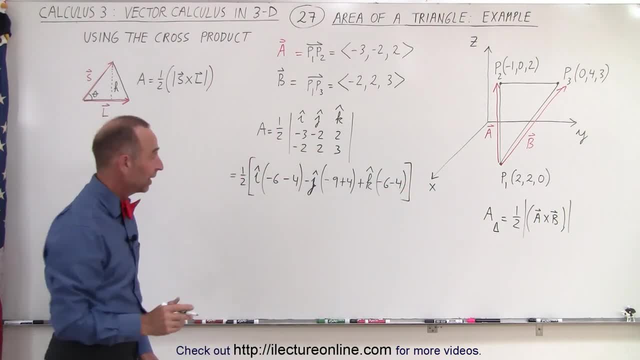 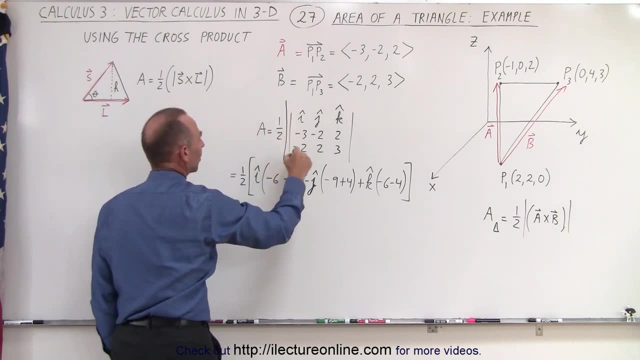 And then I need a bracket around it All. right now let's simplify that. So this is equal to: oh and remember, the area will be the magnitude of this. So of course, I need to put absolute value signs around it like this: 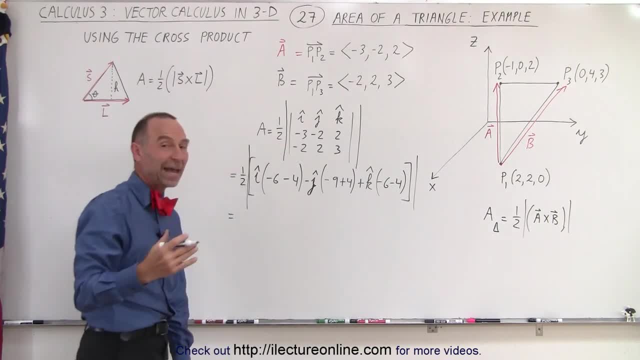 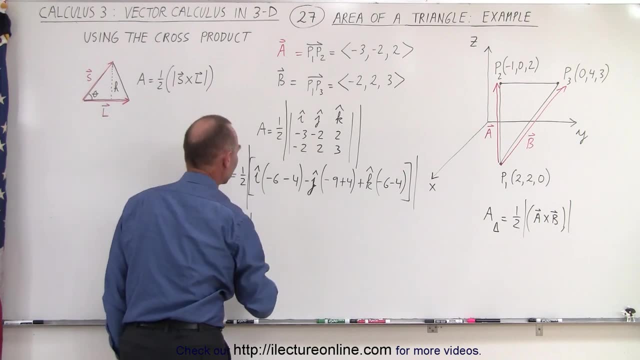 and put absolute value signs around it like this, because I'm actually looking for the magnitude, not the actual cross product. So this is equal to one-half times negative, 6 times negative, 4, that's a negative 10 in the I direction. 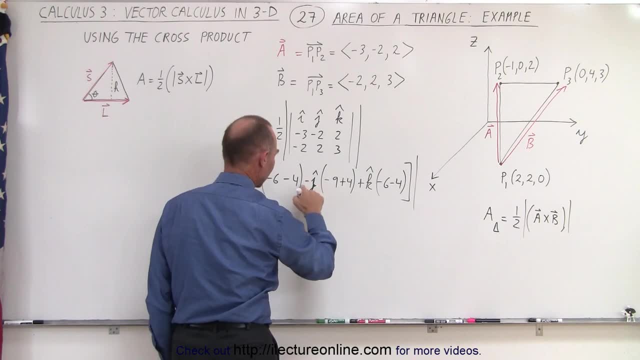 We have minus 9 plus 4, that's a minus. We have minus 5, but with that negative there it becomes a plus 5 in the J direction and that would be a minus 10 in the K direction. Of course, again, I need the absolute value of that. 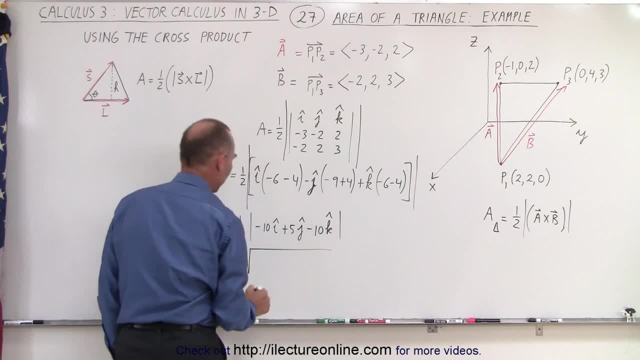 So this is equal to one-half times the square root of the sum of the squares of the components, which is 10 squared plus 5 squared plus 10 squared. Of course, since I'm squaring, I don't care about the negative signs. 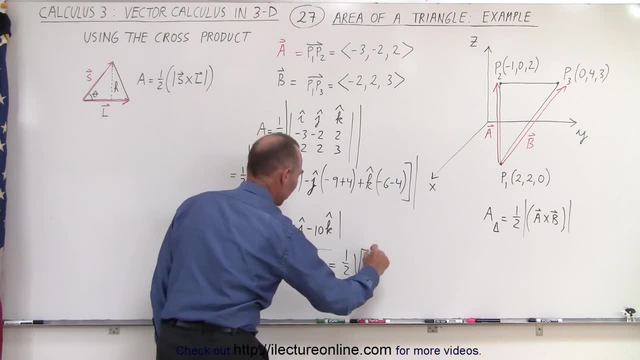 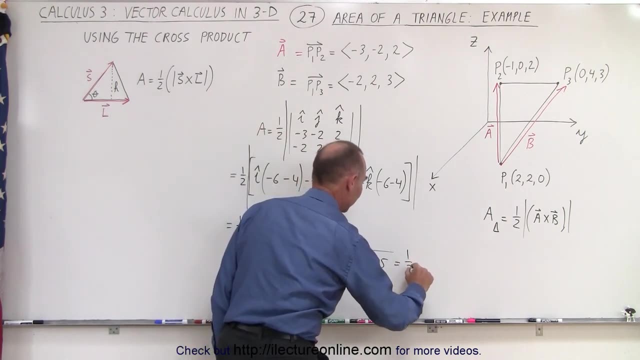 So this is equal to one-half times the square root. the square root of 100, 225, and the square root of 225 is 15, so that's one-half times 15, or 15 divided by 2.. And there you go.